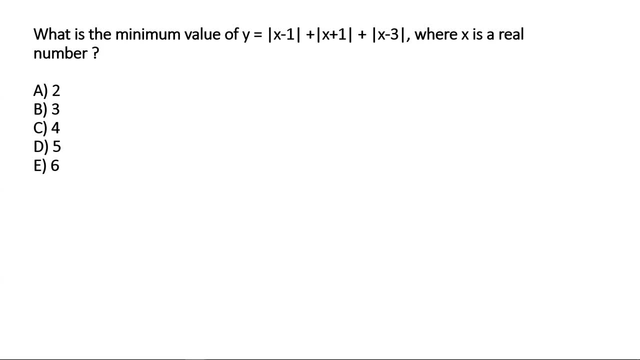 Where x is a real number. So these problems are common in a number of standardized tests. that involves the modulus sign or the magnitude sign or the absolute values, And these are actually not hard to deal with, but it helps to find a method that can be. 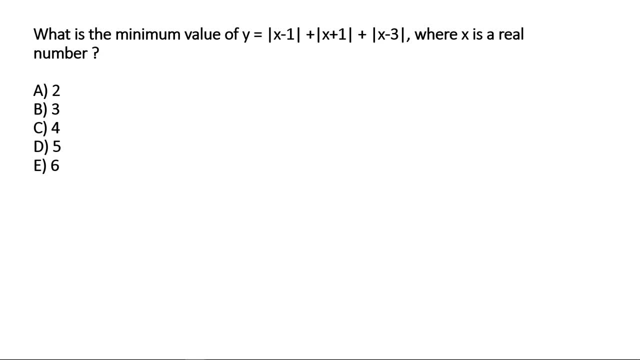 applied to solve such problems in a system that leads you to a correct, reliable answer. So, first of all, we start with this definition of how, in a modulus of a variable, or you could call it the magnitude or the magnitude function, or the absolute value function of a variable, 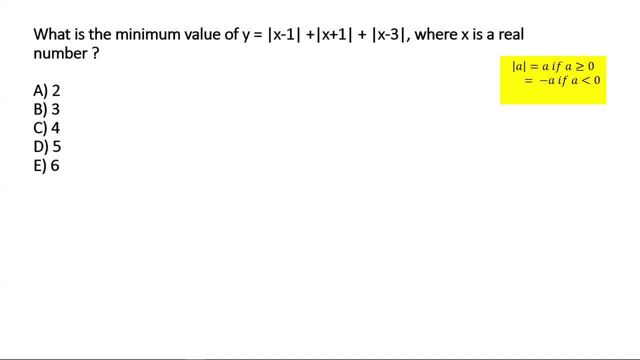 is defined and it's usually written by two bars on either side of the variable. so that's the modulus of a and that is equal to a if the value of a itself is a positive quantity rather than equal to zero, whereas if a has a negative value less than zero, then the modulus 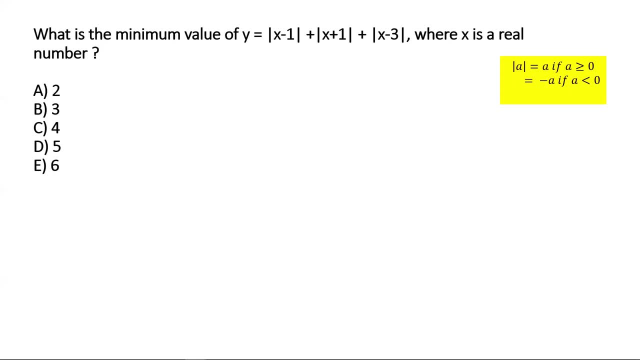 of a will be simply negative a, And to describe it, This is basically, you know, just the magnitude of the variable without the sign. so that's what modulus of a variable essentially means. So now we are given this function, y, which is basically the sum of absolute values of 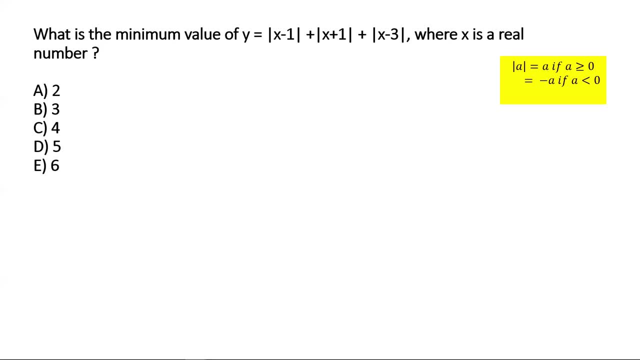 three variables and all of these variables are in x, so there are x minus one, x plus one, x minus three. so we will basically, you know, start by paying attention to the terms within the modulus sign, So each of those three terms within the modulus sign and basically you know defining this. 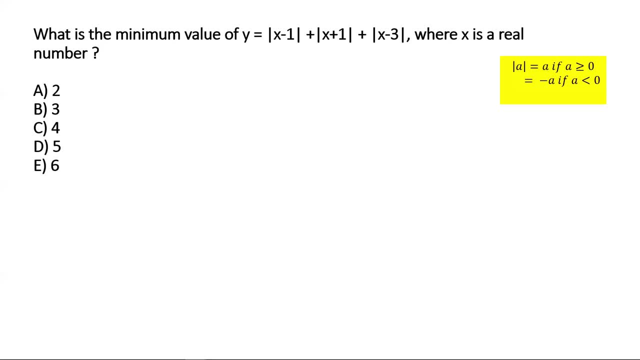 function y, you know, depending on how the signs of those individual variables within the modulus sign changes. So let's start with this one. So here we have x minus 1,, x plus 1, and x minus 3.. So those are the three variables within the modulus sign. 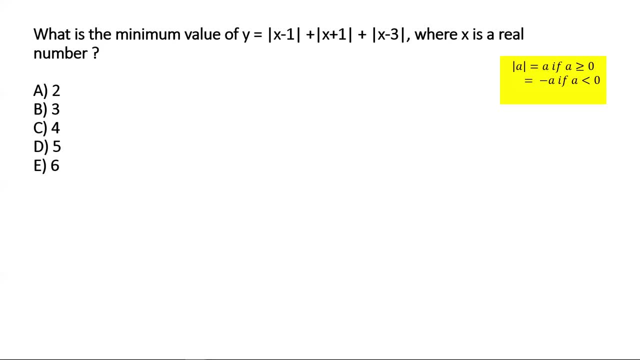 So let's start with what happens when x is less than minus 1.. Then it turns out that each of those three terms within the modulus sign are negative And the value of y will be therefore minus x plus 1.. So we're basically taking the negative of x minus 1.. 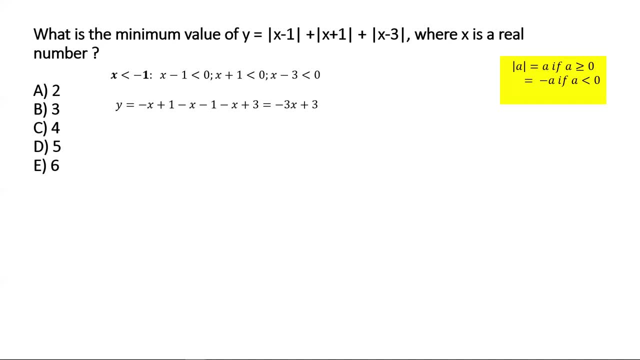 So that becomes minus x plus 1.. Then x plus 1 becomes minus x minus 1.. So that's just the negative of x plus 1, within parentheses right. And then x minus 3 becomes minus x plus 3.. The modulus of x minus 3.. 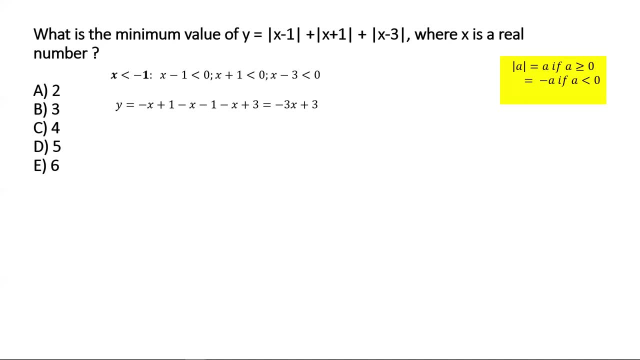 In this case it will be minus x plus 3.. Because all of those three quantities, you know, they are less than 0. So their modulus will be basically the negative right, And now we can simply sum this up And that sum comes to minus 3x plus 3.. 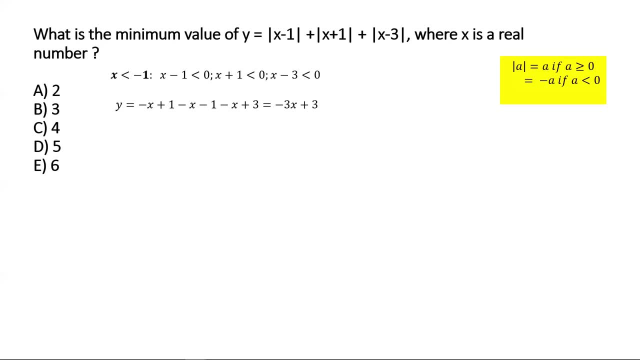 So whenever we have a linear function, it's a linear one-variable function, right, And the sign before the variable is negative. In this case it's x. The sign before x is negative, So that means that this is a decreasing function. 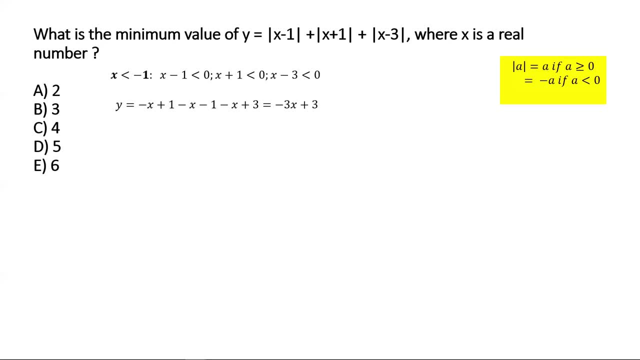 This is a function with a negative slope right And we know that for functions with negative slopes they're decreasing functions and lesser the value of the variable right, Greater is the value of the function And, conversely, Greater the value of the variable, lesser is the value of the function. 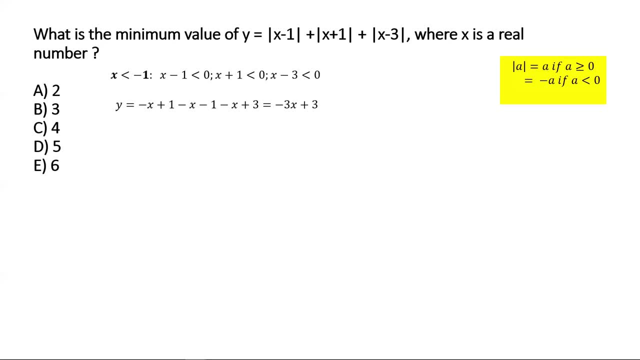 And then, lesser the value of the variable, greater is the value of the function. So if we are to find the minimum value of minus 3x plus 3, and remember that here x, we're only considering values of x less than minus 1.. 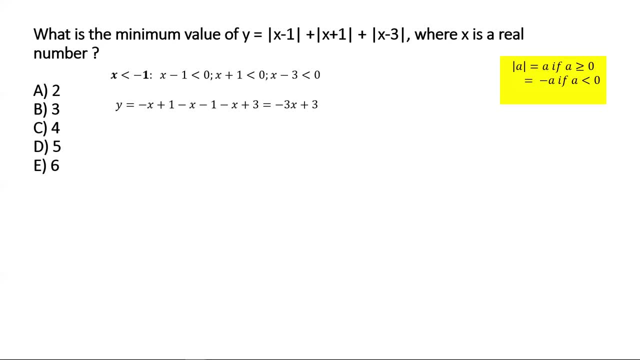 So this is defined only for values of x less than minus 1.. Since this is a decreasing function, this function will take its minimum value at the highest point. So this is the highest possible value of x within the range. Now, as x becomes more and more negative, 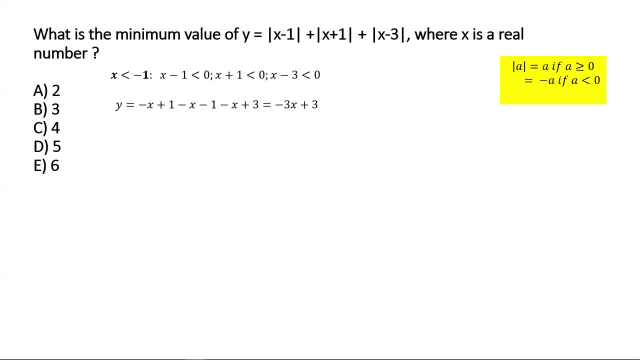 so if it goes from minus 1 to minus 2 and minus 3, the value of this function will basically increase because it's a decreasing function. So as the value of x decreases, the value of y will increase because of that. So if we are to consider what's the minimum possible value of this function, 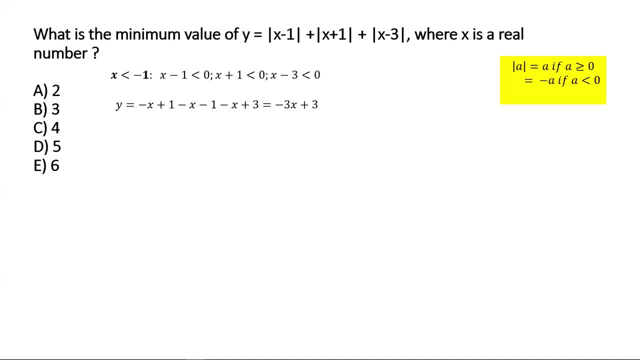 of course, within the range of x right. so this is only defined, remember, for x less than minus 1.. So this is a decreasing function and if you have to find out what's the minimum value of this function, since this is a decreasing function, we have to find the minimum value. 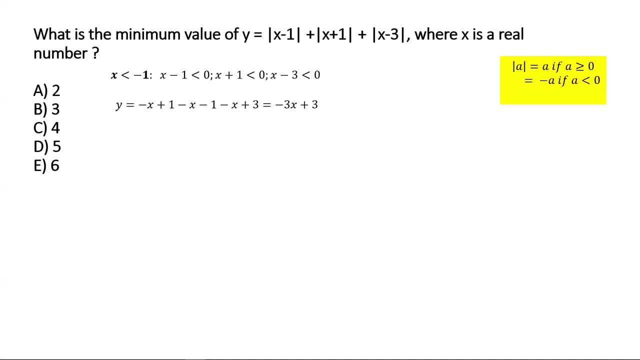 at whatever the maximum possible value that x can take. And since x is less than minus 1, the maximum possible value that x can take is x minus 2.. value that x can take within this definition, within this range, is close to minus 1.. So 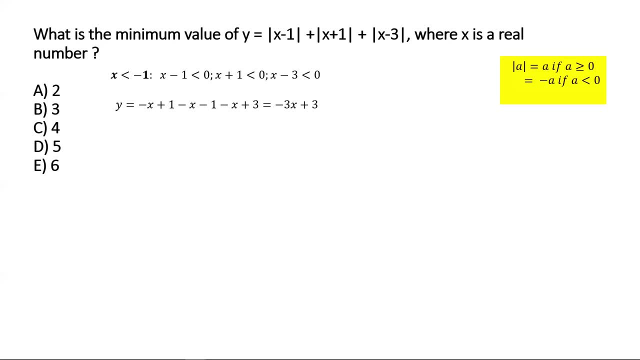 we do not have a, you know, less than equal to sign, So less than sign. So it is x can take its maximum possible value close, something that is very close to minus 1.. And if that happens, then the value of y will be the minimum possible value within this range, right? 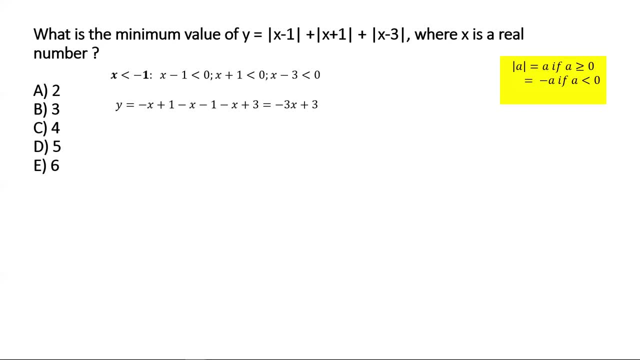 And that will basically I write the tending to, So I cannot write a strictly equal to, because we have x less than minus 1 and not x less than equal to minus 1.. So the minimum value of y will basically be tending towards the value that this function will take when x. 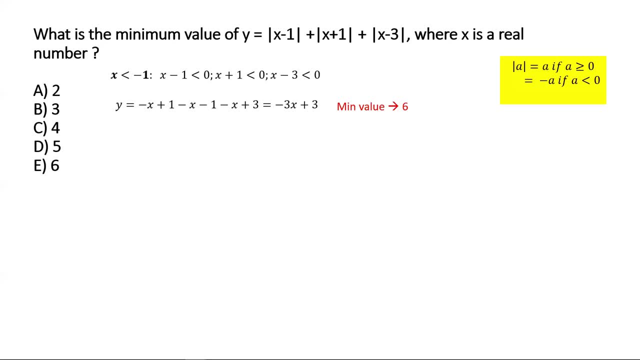 you know, is very close to minus 1, and that will be So. if you substitute x, equal to minus 1, in minus 3, x plus 3, you basically get, you know, minus 3 multiplied by minus 1, which becomes positive 3, and then 3 plus 3.. So that makes 6.. So that is the minimum value. So the minimum. 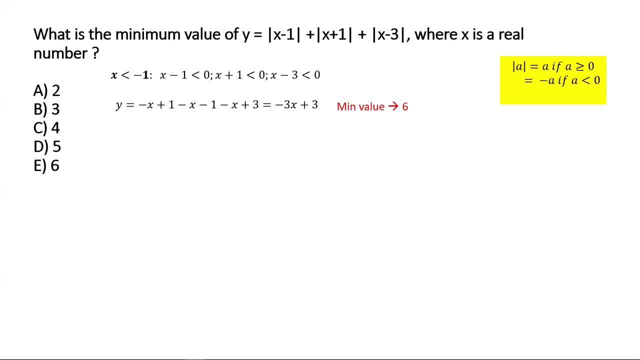 value within this definition is, you know, something that is very close to 6, if not equal to 6, right? So let us consider some of the other ranges. What happens when x lies between minus 1 and 1.. So minus 1, you know, less than equal to x, less than 1.. So that is the range of x In this case. 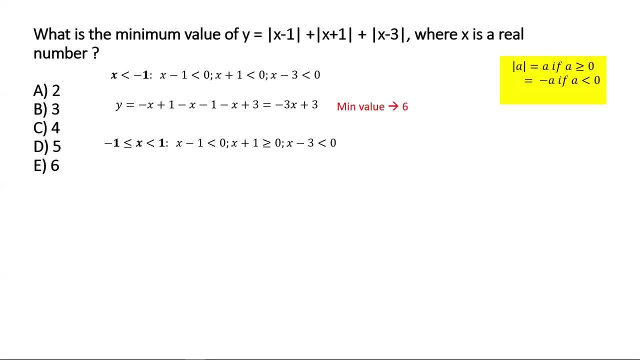 the first term within the modulus, x minus 1, will be less than 0, but the middle term, x plus 1, will be actually greater than equal to 0. And then the third term, x minus 3, will be less than 0 and accordingly we can, you know, write the function y as you know: minus x plus 1 plus. 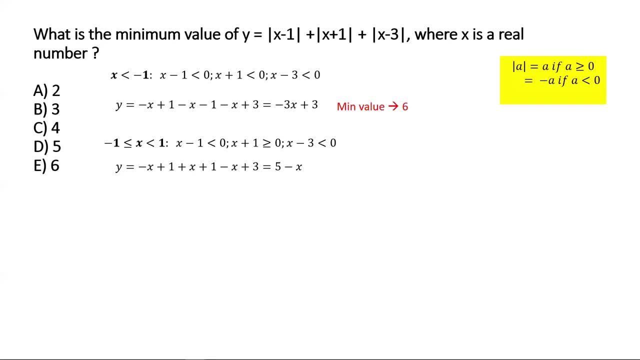 x plus 1 minus x plus 3.. So we just take out the modular sign and, keeping in mind the signs of the modulus, we basically take the value of the variable itself or the negative value and we sum this up and this is what we get: y equal to 5 minus x And again the 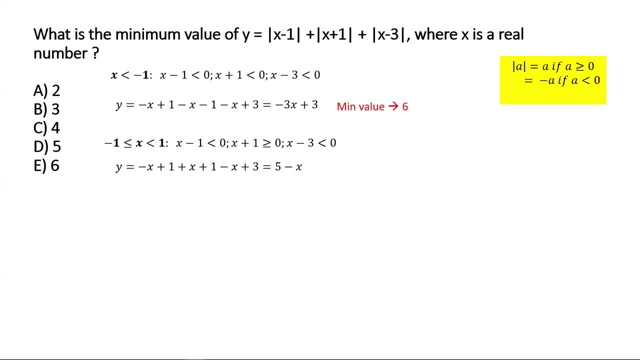 negative sign before x tells me that this is also a decreasing function, meaning higher the value of x. you know, lower is the value of the function. And then we have to ask: well, what is the maximum possible value that x can take within this range and that value? 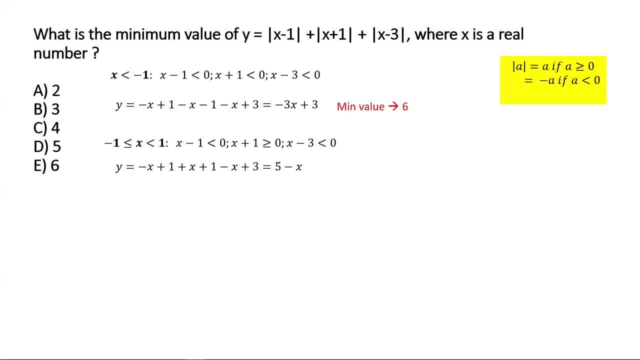 is. you know what is the maximum possible value. So for the maximum possible value, this function, being a decreasing function, will basically take the lowest possible value. So in order to find the lowest possible value of this function, we have to find out the 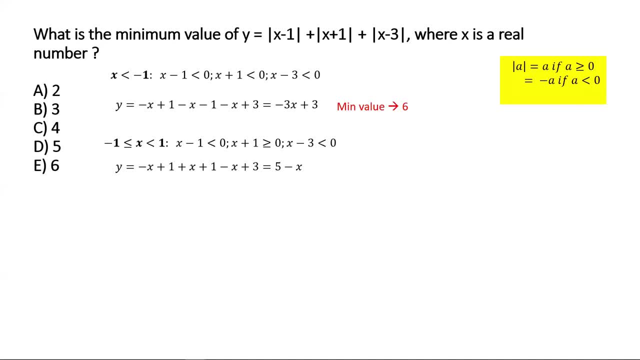 maximum possible value of this function. So we can basically ask what is the maximum value of x? and since x is defined, the range is defined is minus 1, less than equal to x, less than 1.. So the maximum possible value of x will be something that is close to 1. 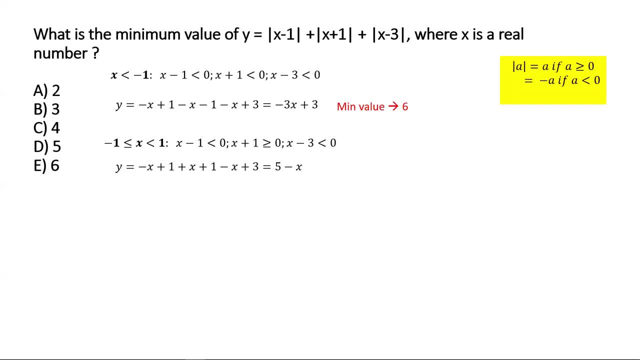 and if we substitute x equal to 1, we can get the minimum value of this function. y will be somewhere close to 4.. So next we consider this range of x, 1 less than equal to x less than 3.. And for this, 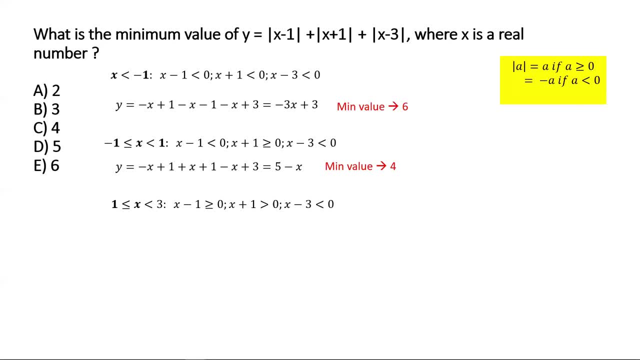 range of x. if you look at the terms within the modular sign, x minus y will be greater than equal to 0, x plus 1 will be greater than 0, but x minus 3 will be less than 0. And accordingly we can write the function. 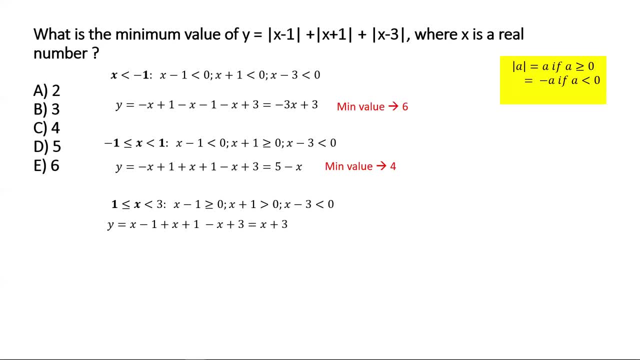 By taking out the modular sign and adjusting the, you know, the signs of the variables within the modulus, and this is what we get: y equal to x minus 1 plus x plus 1 minus x plus 3.. And then if we, you know, do all the addition and subtraction, we basically are left with 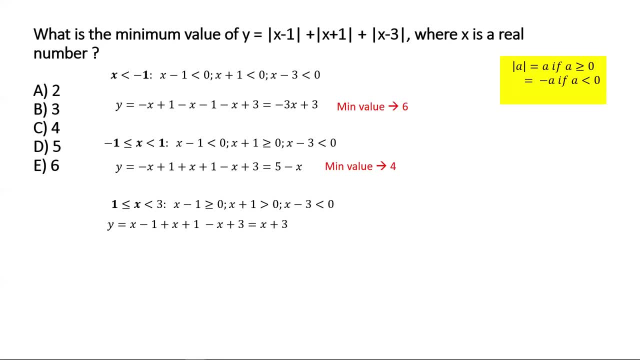 y equal to x plus 3.. So for this function within a range, you have to basically find what is the lowest possible value of x within the range. And in this case the lowest possible value of x within this range is 1.. So this function, y, will take its minimum value for x equal. 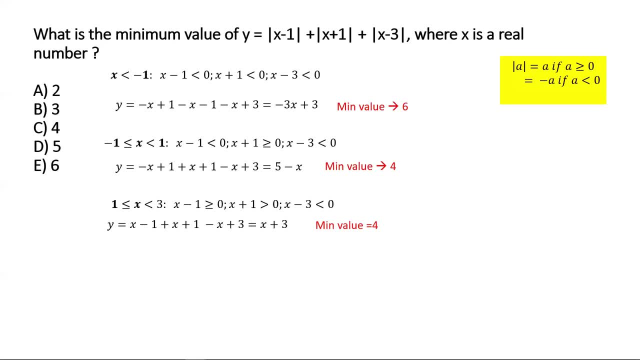 to 1, and that minimum value is going to be equal to 4.. Because the range here, as defined, is 1 less than equal to x. So we can basically, you know, apply the equal sign here, And then there is just one other range of interest for x, which will basically complete. 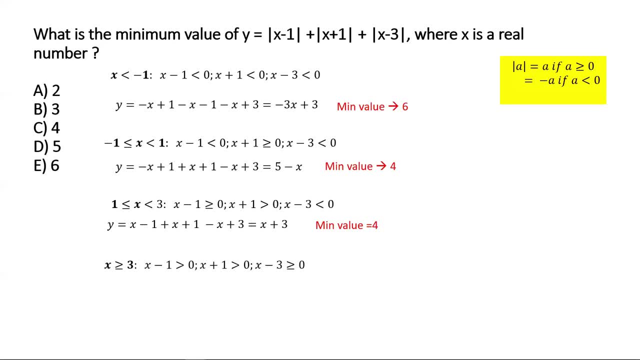 the function definition for all possible ranges of the variable, that's x greater than equal to 3, in which case all of those terms within the modulus are positive. So the value of y will be simply adding those terms up by removing the modulus sign, and that comes to. 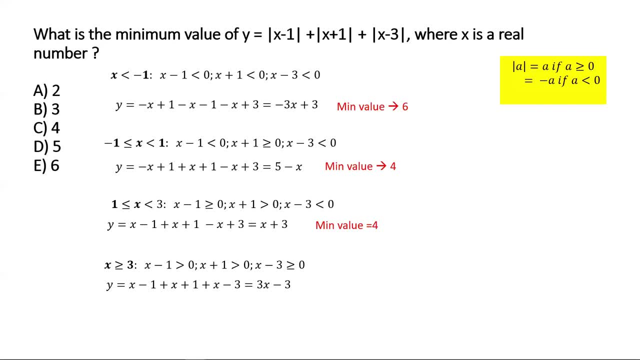 3, x minus 3.. the sign before x is positive here. so this is also an increasing function and we know the increasing function. its lowest possible value, the minimum value, will be also for the lowest possible value of the variable x within the range. in this case that value is 3, so the minimum value of this,